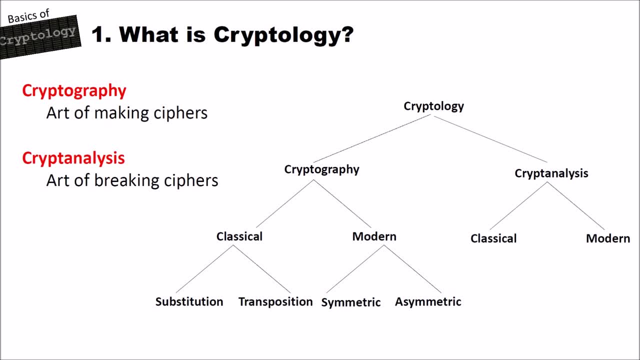 which is done with modern computing techniques. Then on the left side, the classical cryptography can be split into substitution and transposition ciphers, And the modern cryptography, or at least the ciphers that we have with modern cryptography, can be split into symmetric and asymmetric ciphers. 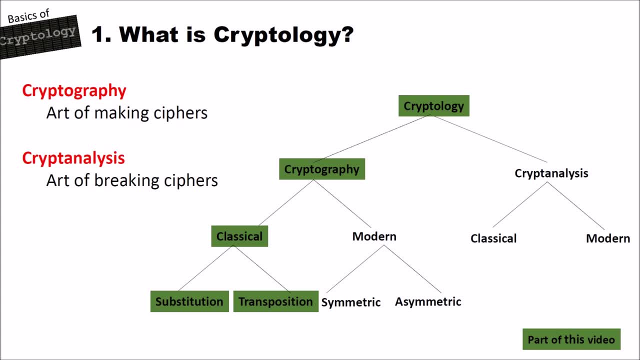 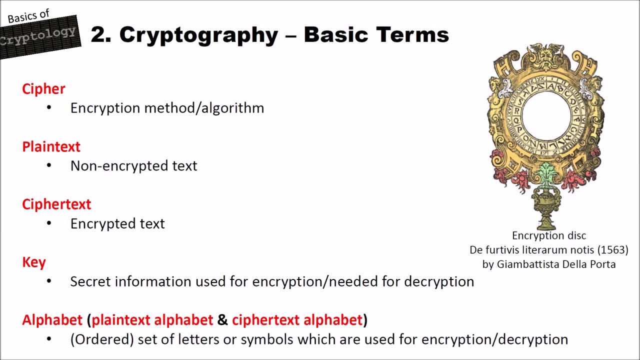 In this video we want to have a look at cryptology, cryptography, classical cryptography and the substitution and transposition. Here are the first basic terms that you will find in every book about cryptology or cryptography. when we speak about cryptography, The first thing is the cipher, And the cipher is an. 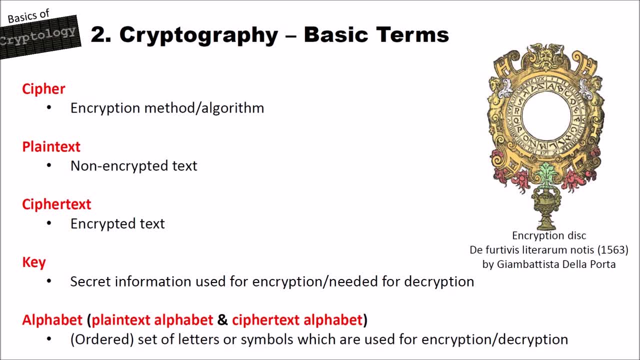 encryption method or algorithm. In many books and papers you also find cipher for ciphertext, but we define cipher only as an encryption method or algorithm. Then we have of course the plaintext, And the plaintext is a non-encrypted text that we want to encrypt. 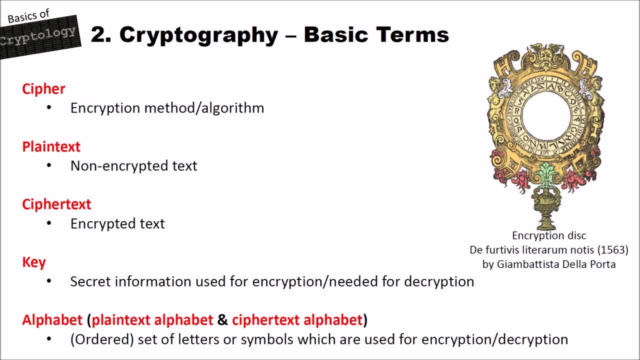 Then we have the ciphertext, which is the result of applying a cipher on a plaintext, And the ciphertext, of course, is encrypted. Then we have the key, And the key is some kind of secret information that is used for encryption and, of course, which is needed for decryption. 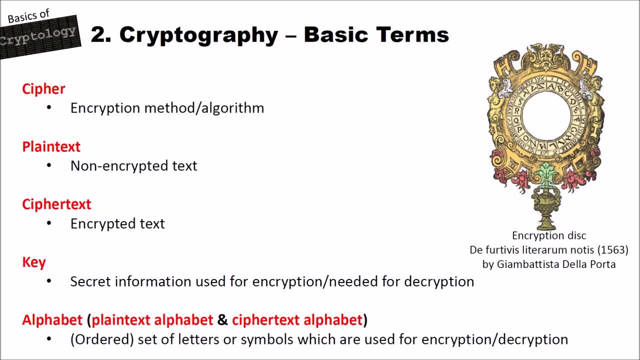 And the key is the only thing that we keep secret. We don't keep the cipher secret and we don't keep how the cipher works secret. So crypto algorithm or method has to be secure by an attacker knowing the complete cipher itself but not having the key. 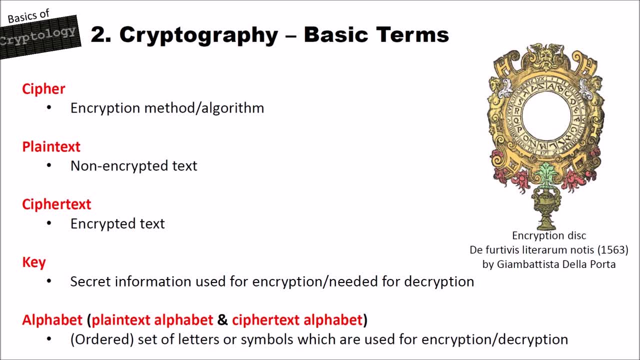 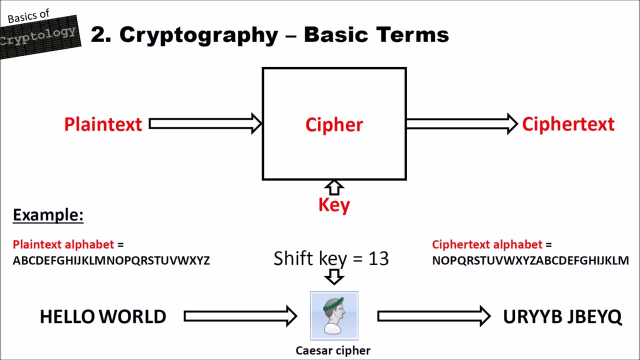 Then we have the alphabet, And the alphabet can be split into a plaintext alphabet and ciphertext alphabet. And an alphabet is an ordered set of letters or symbols which are used for encryption or decryption. Here I try to show how all these words are connected. 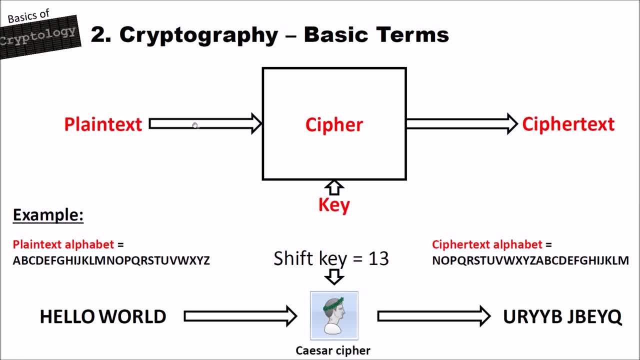 So, as you can see here on the left, the plaintext goes into the cipher. Also, the key goes into the cipher. The cipher then performs a method or an algorithm on the plaintext with the help of the key, And the result of the cipher then is the ciphertext. 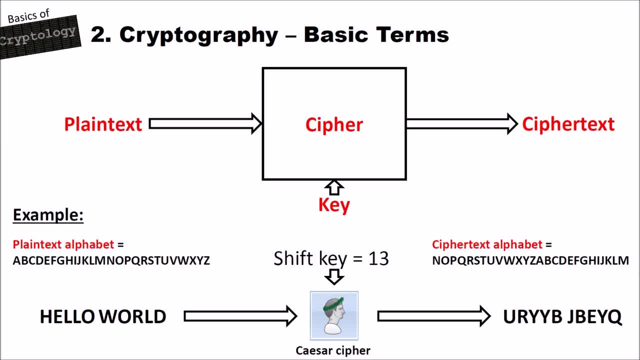 Here is a short example for a real-world cipher, In this case the Caesar cipher On the left side. you see here the plaintext alphabet that is used with Caesar. It's a latin alphabet from A to Z. Then we have a plaintext message here which is: hello world. 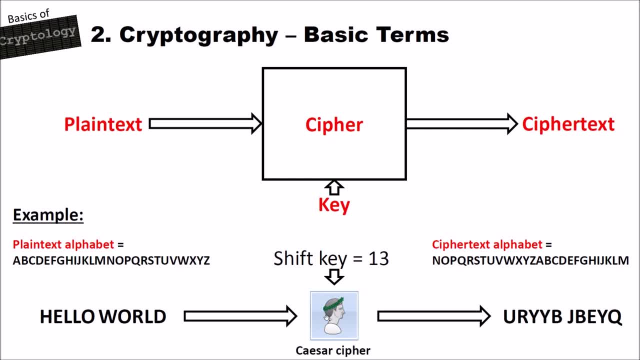 In the middle we have the Caesar cipher that we use for encryption, which also needs a key. In the case of the Caesar cipher, it's a shift key And its value is 13.. So it's a shift key. If you are further interested in the Caesar cipher, I already made a video about this. 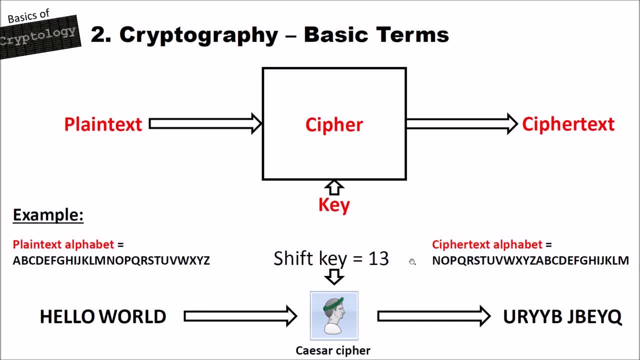 So you may have a look at this. And here on the right side we now see the ciphertext alphabet, which is shifted by 13. So it doesn't start at A, it starts at N and it doesn't end with Z, it ends with an M. 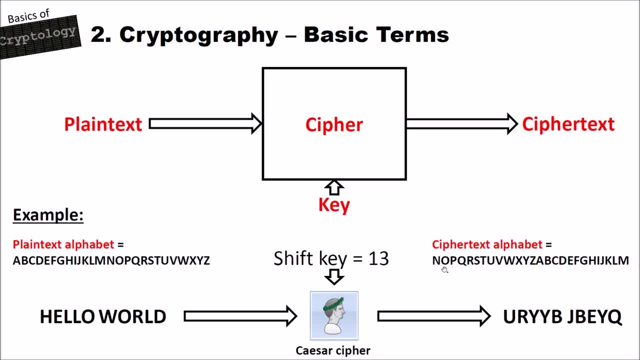 So the A is encrypted to N, the B is encrypted to O, and so on and so on, and the Z is encrypted to M, And the result, of course, of the Caesar cipher is the ciphertext here, Which is U R, Y, Y, B, J, B, E, Y, Q. 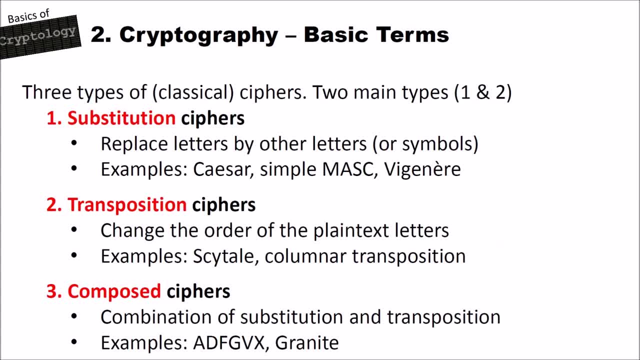 There are three types of classical ciphers: Two main types and an additional one. The first main type is the substitution ciphers type, And substitution ciphers replace letters by other letters or, for example, symbols. An example for a substitution cipher is the Caesar cipher or the simple mono-alphabetic. 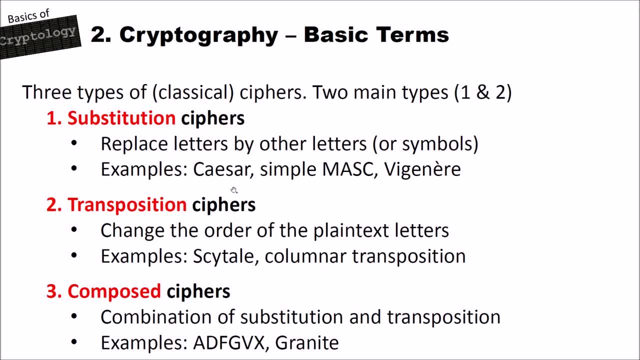 substitution cipher. We already had videos on all these three, So you may have a look at the classical cipher series on this channel. Then we have the second type of ciphers, which are the transposition ciphers. These change the order of the plaintext letters. 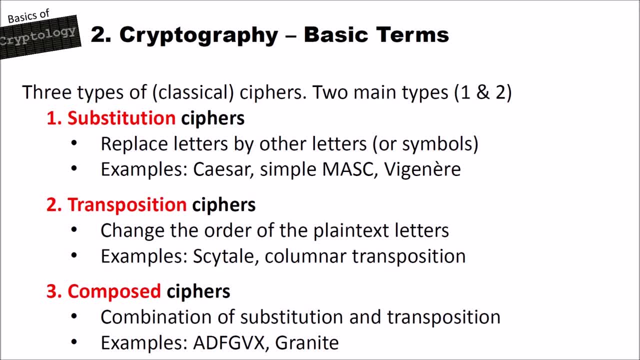 But the plaintext alphabet is the same as the ciphertext alphabet, then Only the position is changed. Examples for this are the citilie cipher or the columnar transposition cipher. We also had videos on these. And the third type of ciphers are the composed ciphers. 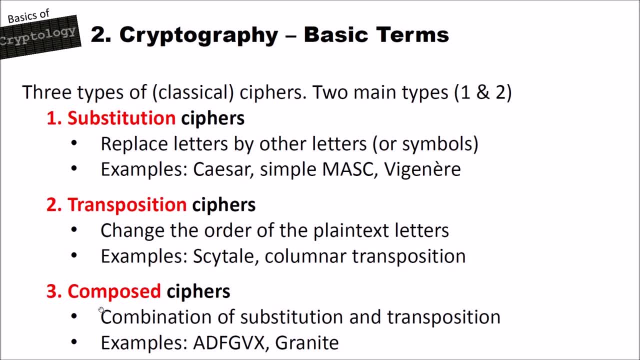 And the composed ciphers are ciphers that are a combination of, for instance, different substitution ciphers or different transposition ciphers, or also a combination of substitution and transposition ciphers. Examples for this are the ADFGVX cipher. We already had a video about this. 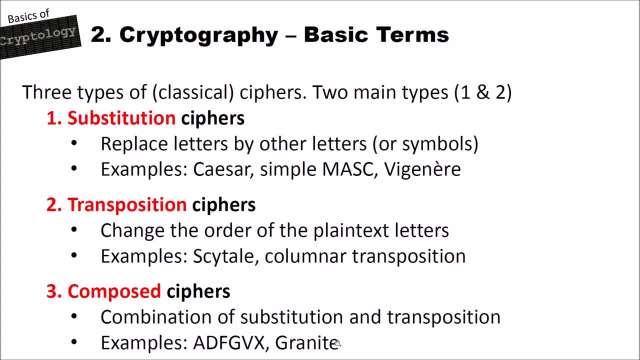 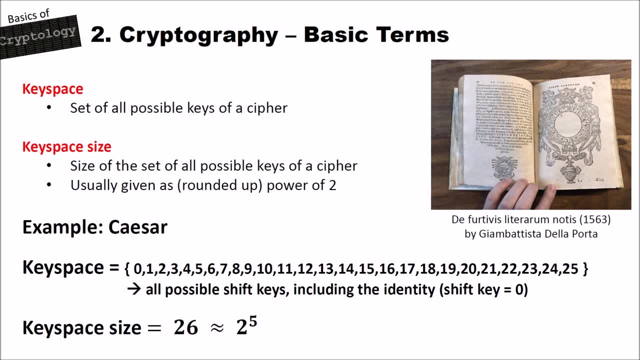 And the Granite cipher, which was used in the Cold War in Germany. Then there are others. There are other important words that we have with cryptography, For instance the keyspace. The keyspace is a set of all possible keys of a cipher, For instance with the Caesar cipher. I have an example here. 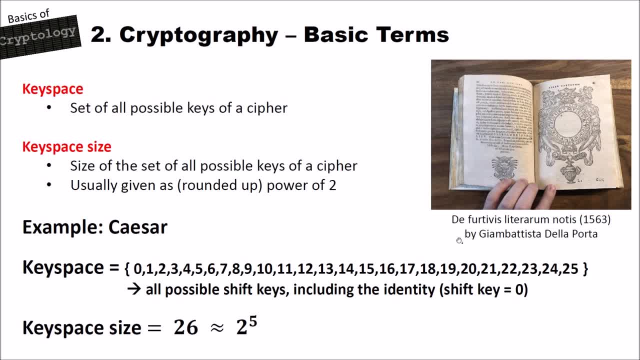 The keyspace are all numbers from 0 to 25.. These are all possible shift values for the Caesar cipher, And the identity, that is, a shift key equal to 0, is also included in the keyspace. The keyspace size, of course, then, is the size of the set of all possible keys of a cipher. 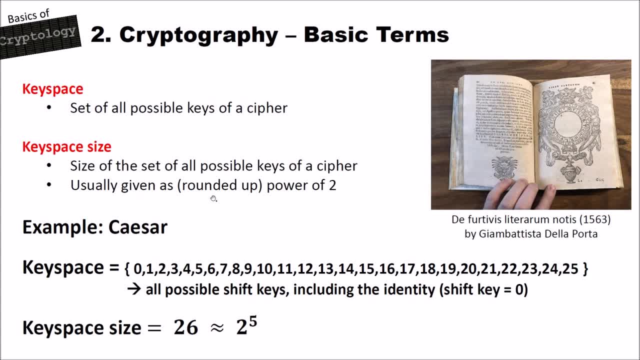 And usually cryptanalysts or cryptographs give these as a rounded up power of 2.. In the case of the Caesar cipher, the keyspace size, of course, is 26, because we have 26 numbers here, and this is about 2 to the power of 5.. 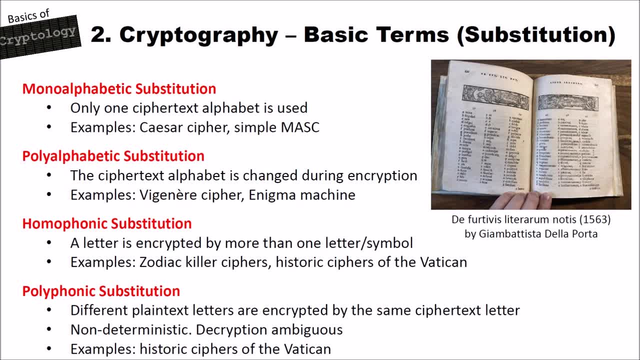 With substitution ciphers, we also have some additional basic terms. First of all, we have monoalphabetic substitution ciphers. The key space size, of course, is 26, because we have 26 numbers here, and this is about 2 to the power of 5.. 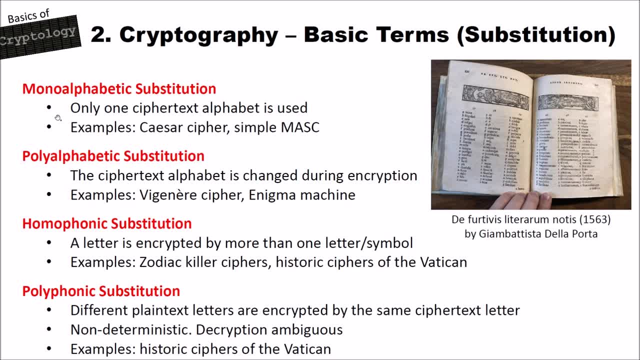 The monoalphabetic substitution cipher only has one ciphertext alphabet. An example for this is the Caesar cipher or the simple monoalphabetic substitution cipher. Then we have the polyalphabetic substitution ciphers And these ciphers- the alphabet is changed during the encryption. 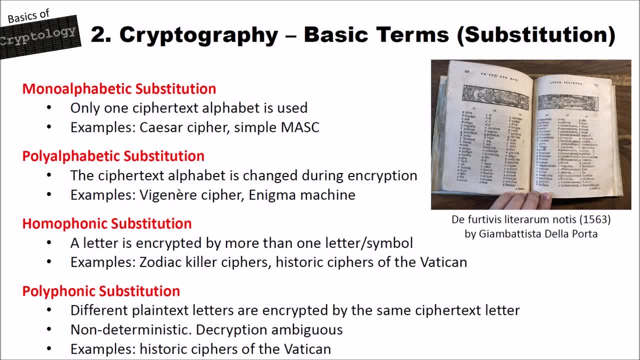 An example for this is the Vigenere cipher or the Enigma machine. With the Vigenere cipher and the Enigma machine we also had videos on this channel so you may have a look at these. Then we have the homophonic substitution ciphers. 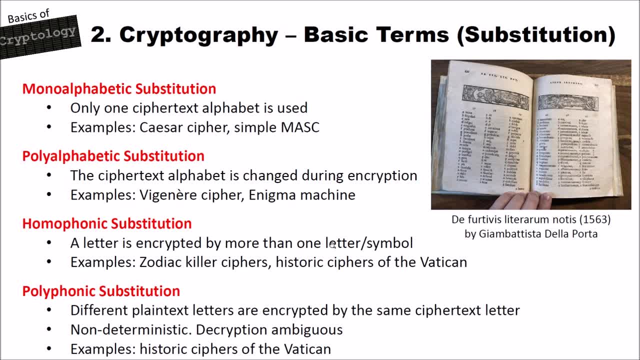 And with a homophonic substitution. a letter is encrypted by more than one letter or symbol. So A is, for instance, encrypted with 01 and 05 and B is encrypted with 09 and 07 and so on. Examples for this are the Zodiac killer ciphers- we also had a video on this- or historic ciphers. 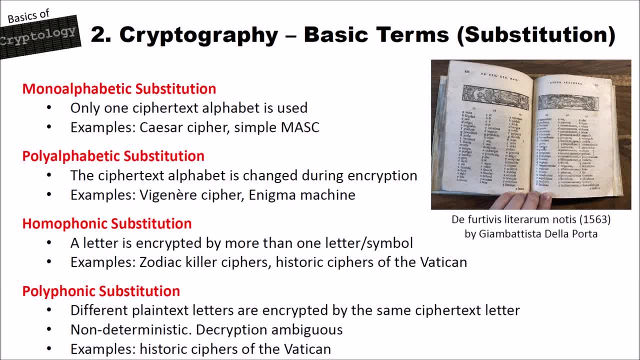 that were used in the Vatican. Then we have polyphonic substitution ciphers And with these ciphers Different plaintext letters are encrypted by the same ciphertext letter. And this makes this kind of cipher problematic, because they are non-deterministic and the 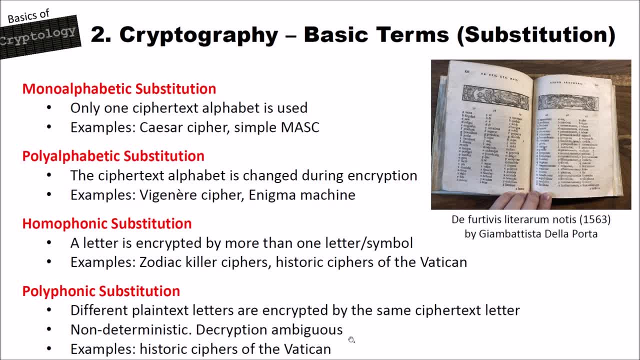 decryption is ambiguous And the problem is: when you encrypt an A with an X and a B, you also encrypt with an X. Then when you have the X in the ciphertext you want to decrypt, you don't know was it an A or was it in B. 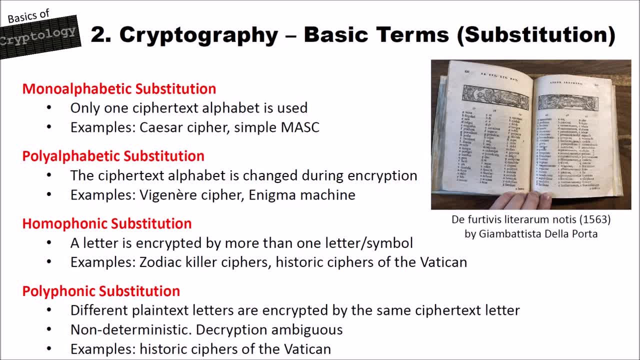 So you need the context of the letter, For instance. So three letters before and three letters after this, and then you know: okay, this can only be an A, And examples for this are historic ciphers that were also used in the Vatican. So we have examples for polyphonic substitution ciphers and they are really hard and difficult. 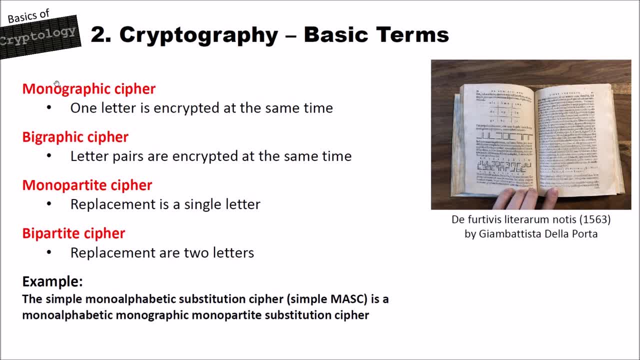 for cryptanalysis. Then we have other basic terms for cryptography. For instance, we have monographic ciphers, And with a monographic cipher one letter is encrypted at the same time. An example for this is the Caesar cipher, where you first encrypt the letter. 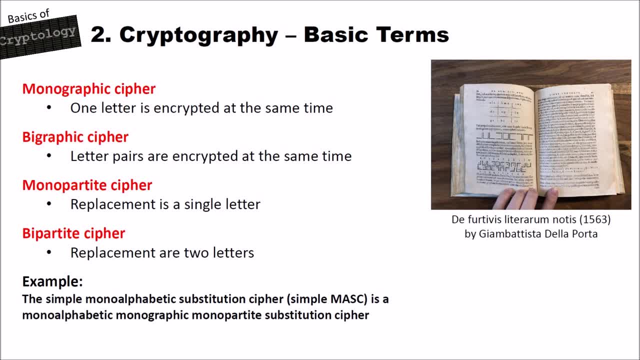 You first encrypt the first letter, then you encrypt the second letter, and so on. Then we have bigraphic ciphers And with bigraphic ciphers letter pairs are encrypted at the same time. So you encrypt the first two letters, then the second two letters and the third two letters. 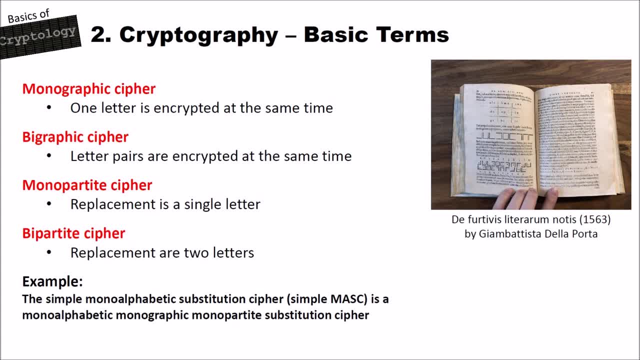 and so on. An example for this is a Playfair cipher, where we also had a video on this channel. Then we have monopartite ciphers and with a monopartite cipher, the replacement of a letter, or maybe monopartite ciphers, is a monopartite cipher. 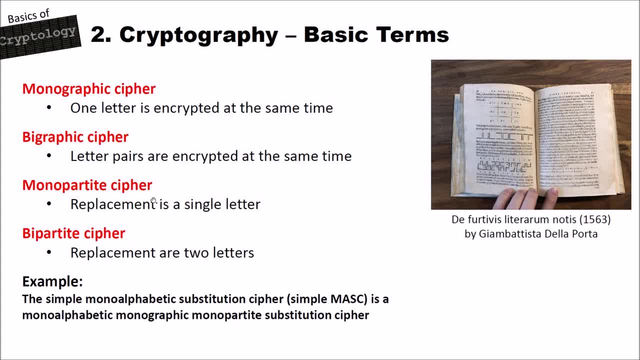 Also the Caesar cipher is an example for this. We replace a single letter with another single letter, And then we have the bipartite cipher, and with the bipartite cipher we replace a letter, for instance, with two letters. An example for this is the ADFGVX, where we first, or in the first step, where we encrypt. 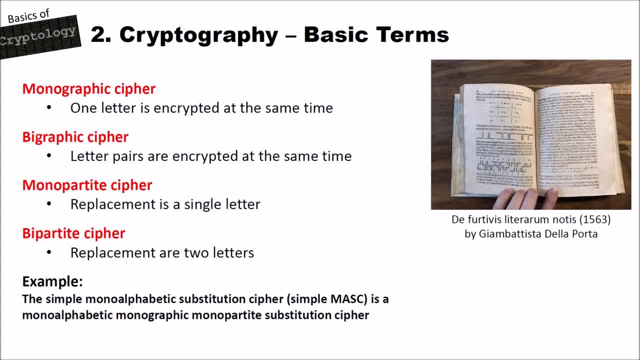 a letter, For instance an A with an DD Or a B with an AX and so on. So we replace one letter by two letters. So the graphic here also refers to the plaintext. So what we do with the plaintext And the partite here also always refers to what we do in the ciphertext. 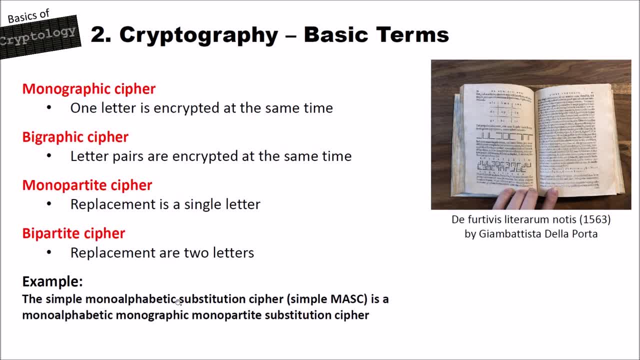 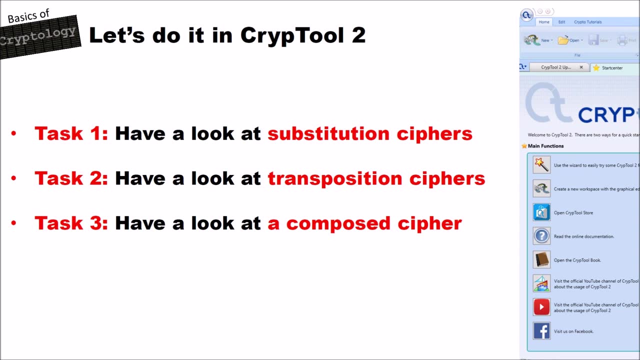 And an example is, for instance, the simple monoalphabetic substitution cipher, or short, simple mask, Which is a monoalphabetic, monographic, Monopartite substitution cipher. So this was everything that I wanted to discuss with terminology. So now we will have a look in Cryptool 2 at substitution ciphers. 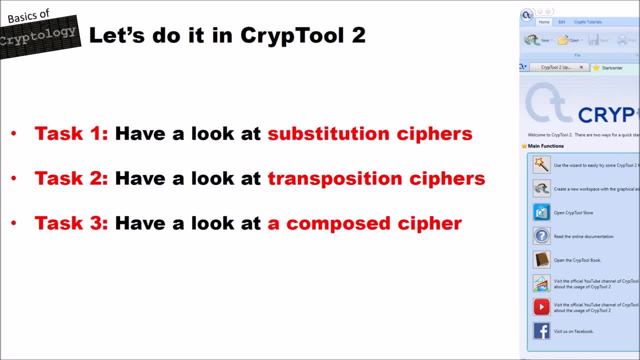 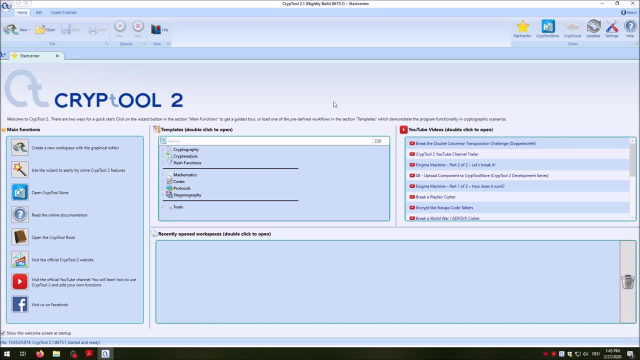 Then we will have a look at transposition ciphers And finally we will have a short look at composed ciphers. I'm here now in Cryptool 2 and I want to first show you some examples for substitution ciphers or classical substitution ciphers. 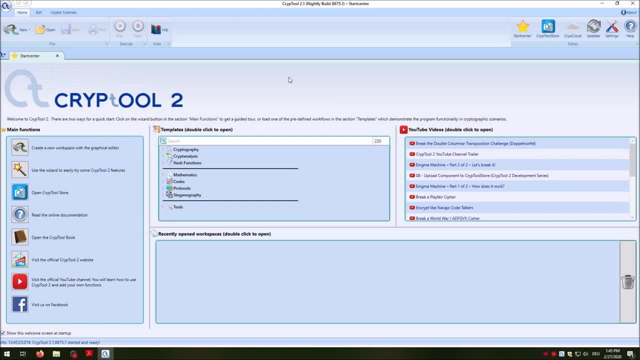 And you find the substitution ciphers by going to cryptography and classical, And here we have substitution and transposition ciphers And the first example for a simple substitution cipher is the caesar cipher. Just double click it and then it opens the workspace. 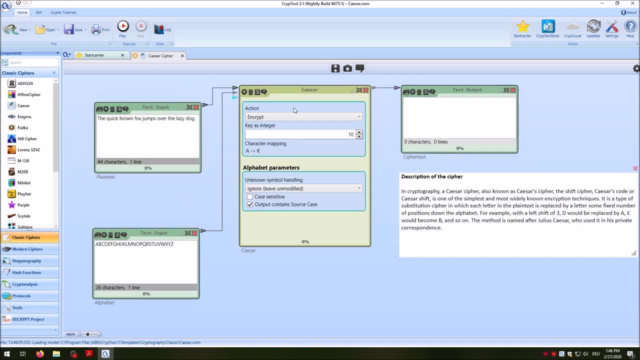 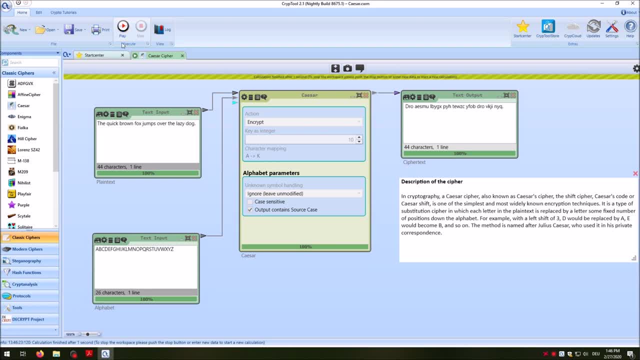 And here is a simple substitution cipher, And to execute it in Cryptool 2, you just click the play button And what do we see here? We have a shift of 10.. So, as I already said, the caesar cipher shifts the alphabet, the plain text alphabet. 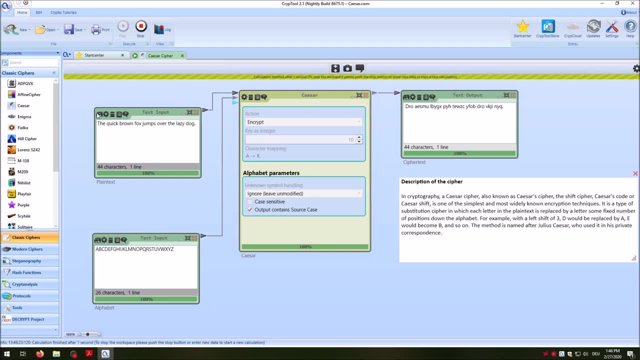 And you can specify here the alphabet that should be used, And, for instance, the t substituted by d, The h by r and so on. And, as always in Crypto2, you can type and it will live encrypt what you are doing. Hello, this is the test of the Caesar cipher. 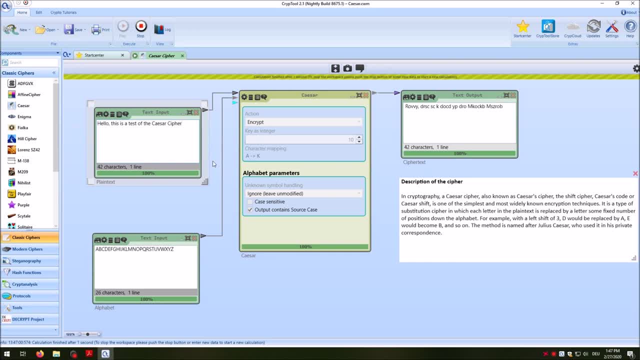 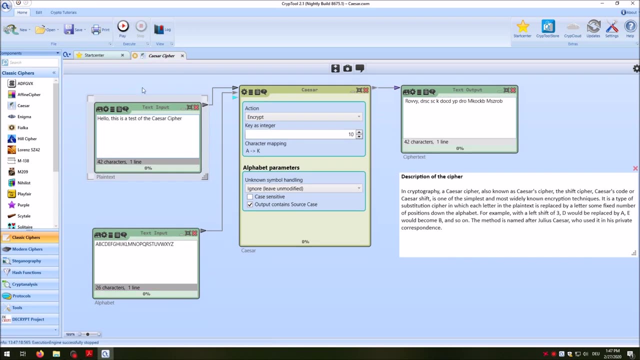 And the Caesar cipher is now set to ignore the. no, it's not set to ignore. it should contain the source case. So if you write lowercase and uppercase, it will encrypt also in lowercase and uppercase. So let's have a look at another substitution cipher. 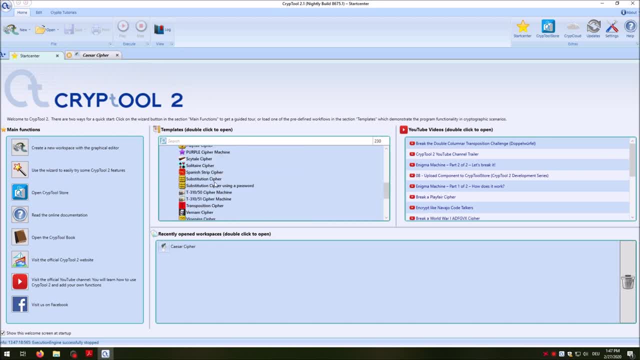 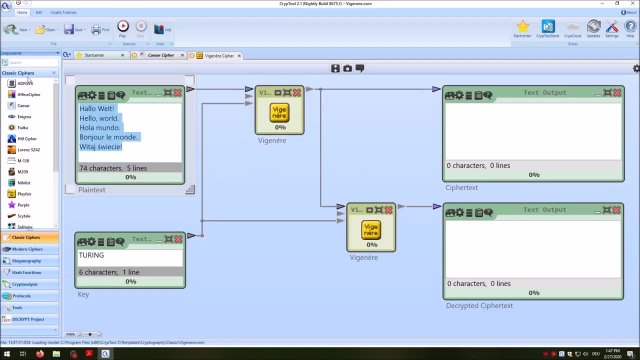 For instance, we could have a look at the Vigenere cipher here. So we just double click the Vigenere cipher and we will write a text: Hello, this is the test of the Caesar cipher. We already had videos about this. 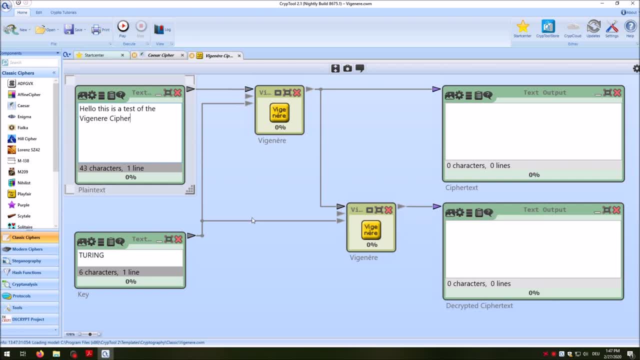 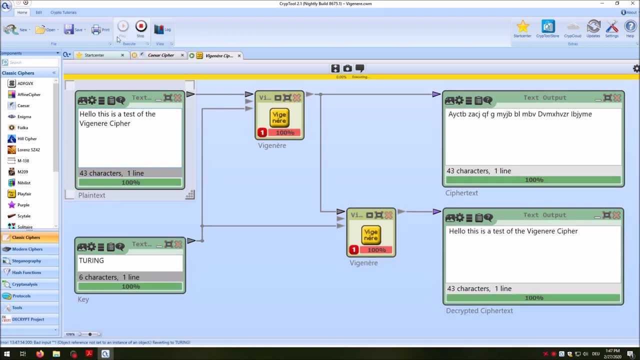 so I don't describe in detail how these ciphers works. So if you're interested in this, you should have a look at the other videos. and of course we have to click play. And then we see here the Vigenere cipher, encryption and the decryption. 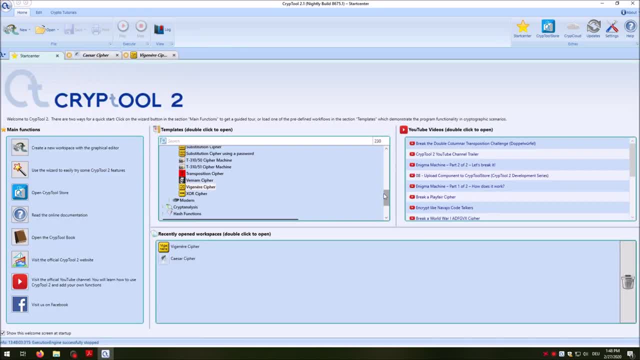 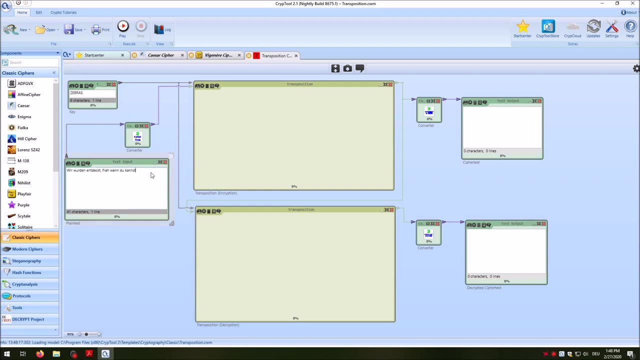 Now let's have a look at an example transposition cipher. For this I go to the columnar transposition. So we have here the transposition cipher, Double click and then we write the transposition cipher. We write hello. this is the test of the transposition cipher. 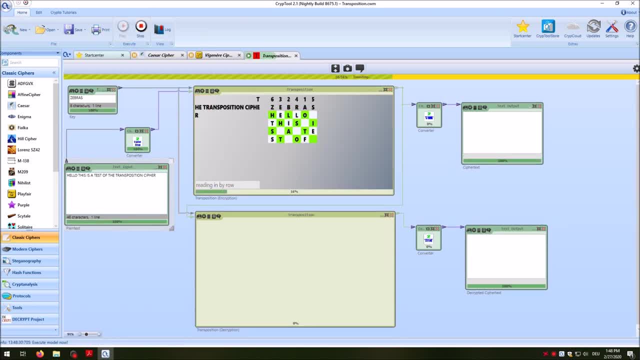 And you also click on play. You can specify the key here, the plain text here. Here you see how the transposition cipher actually works. We also made a video about this so you could have a look at this video. And here we have the decryption of the transposition cipher. 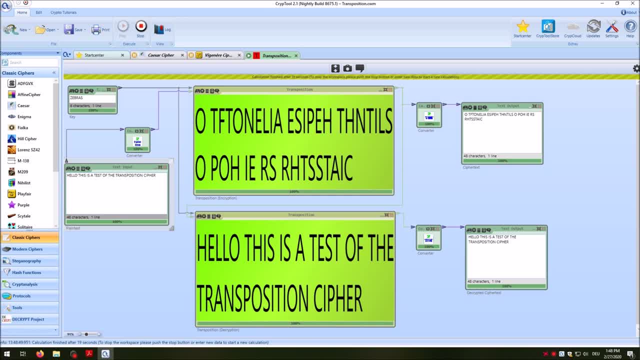 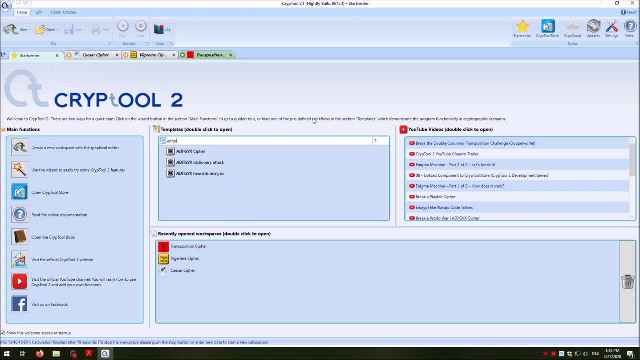 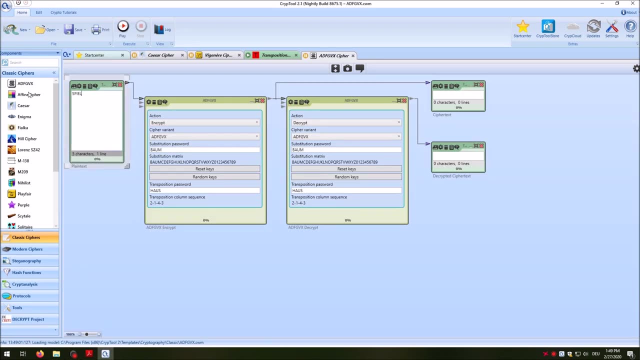 Here we have the cipher text, and here we have the decrypted cipher text. So let's have a final look at a composed cipher. For that we have the ADFGVX And we just open this here And we have our plain text here. 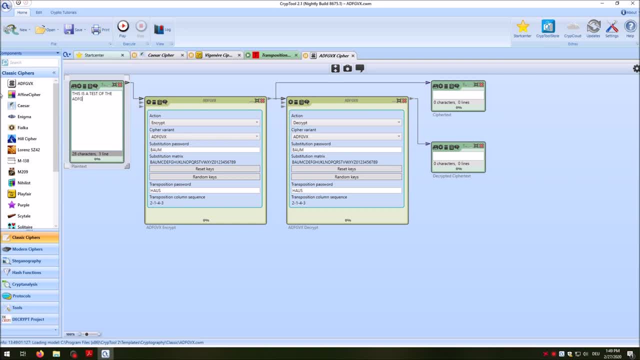 This is the test of the ADFGVX cipher. We also had a video about the ADFGVX, So for details, please have a look at this video And the ADFGVX cipher we have here. And the ADFGVX cipher, as I said, is a composed cipher. 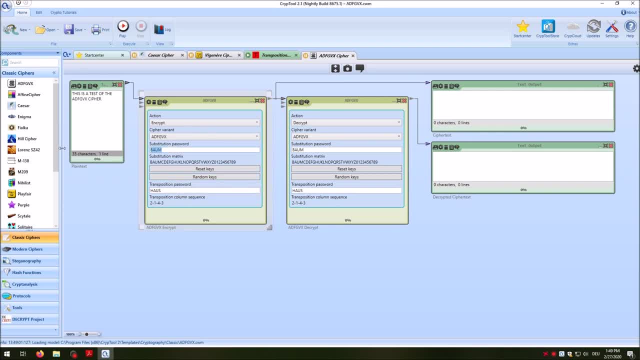 So it needs a substitution password. This is substitution and the transposition password or key or password transposition. And we copy this also to the second component, ADFGVX component, because this decrypts. We have here encryption and decryption. 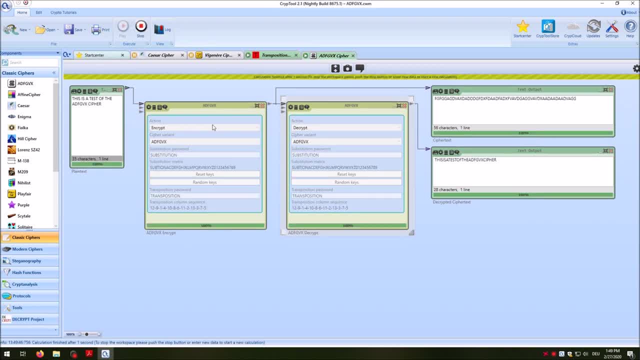 And let's test it. So at first it first uses a substitution to substitute the text, Then it transposes the text, And then we have here the cipher text, which only consists of ADFGVX, And of course the decryption here. 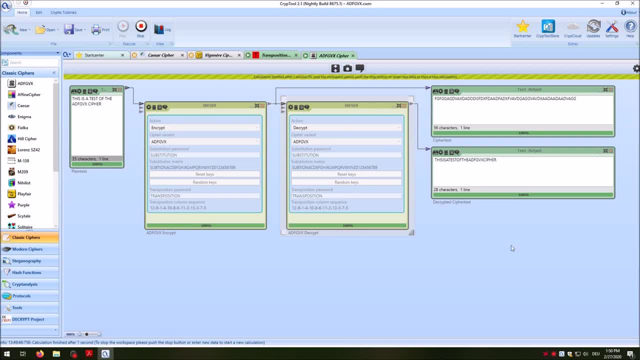 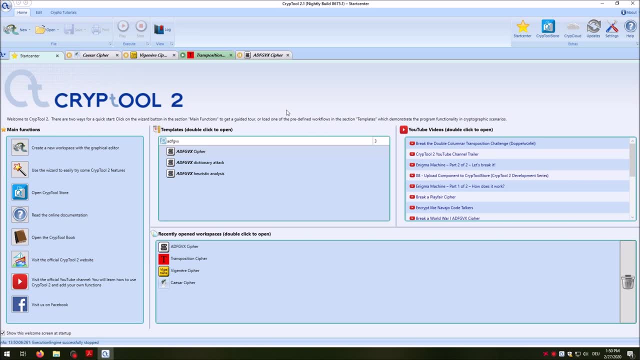 This is a test of the ADFGVX cipher. So in this video I showed you the basic terminology of cryptography, And the cryptanalysis part will be in the next video. There I will show you different attacks on the ciphers and the terminology of cryptanalysis. 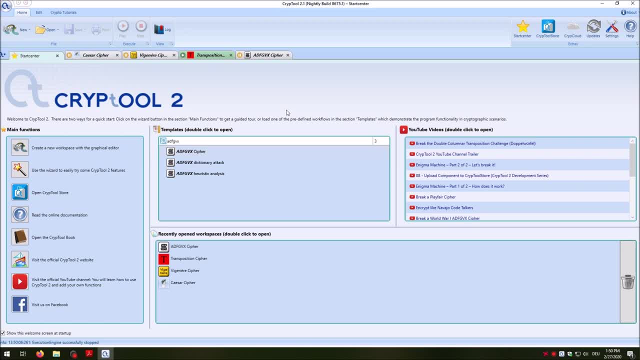 And I hope you liked this video. If you do, please give a thumbs up, And if you're not yet subscribed to our channel, I would be really happy if you subscribe to our channel And see you in the next video.